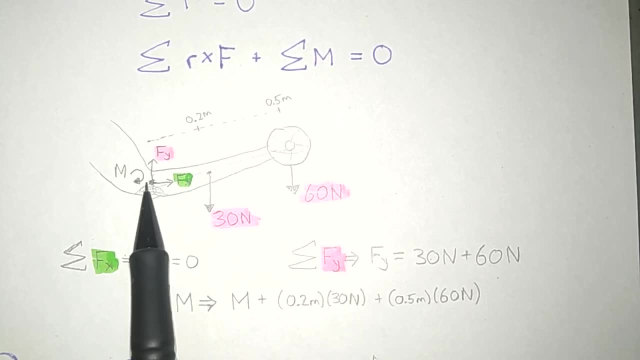 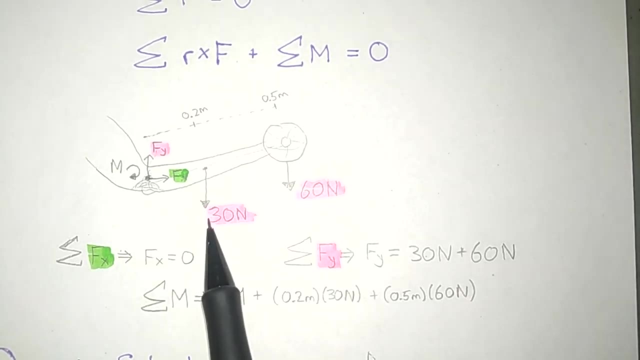 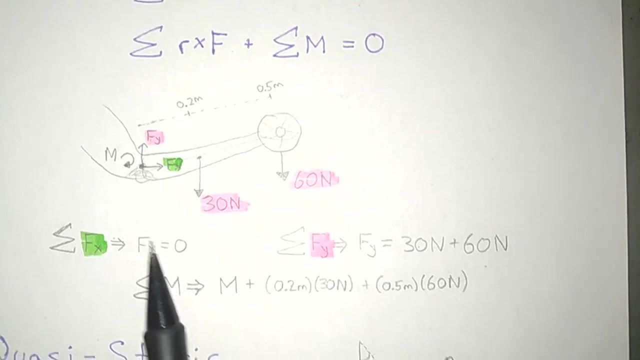 The force of y must be zero. So at this joint there's going to be some force being applied and that must be equal and opposite to the other forces. So we see there's 30 newton here and 60 newton here, which means the force in the y direction must be 90 newtons. 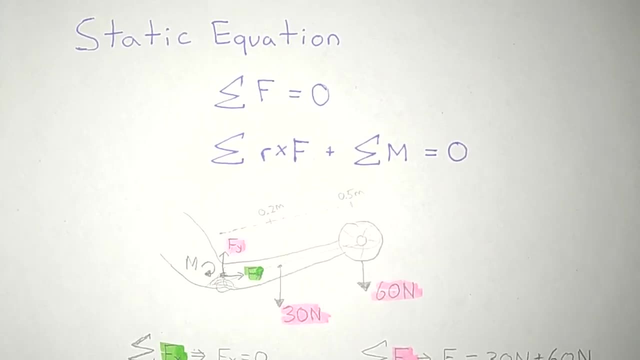 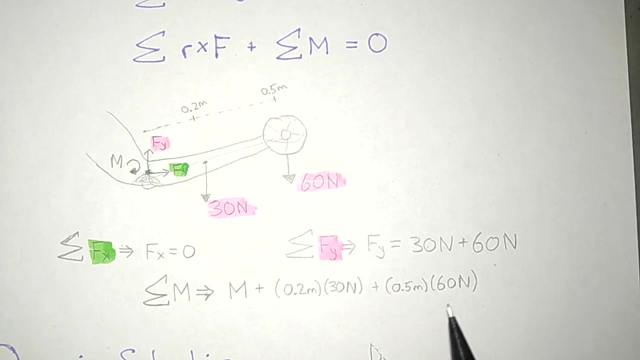 But also notice that the moment must also be zero. The moment across any point must be zero, And to resist that moment there must be some internal moment at this joint that's resisting it. And so we just calculate what is the moment of the circuit that we know. sorry for the diagram that we know. 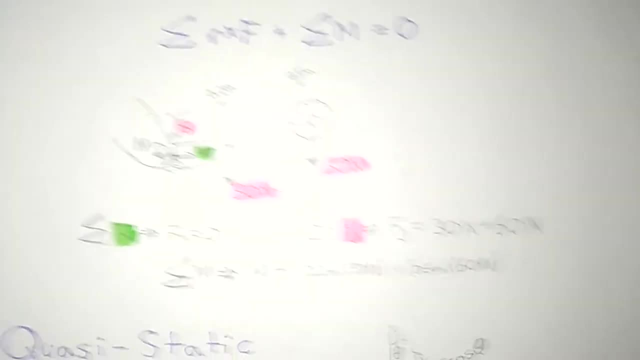 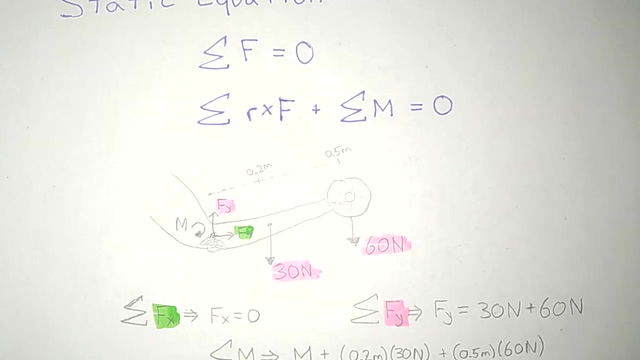 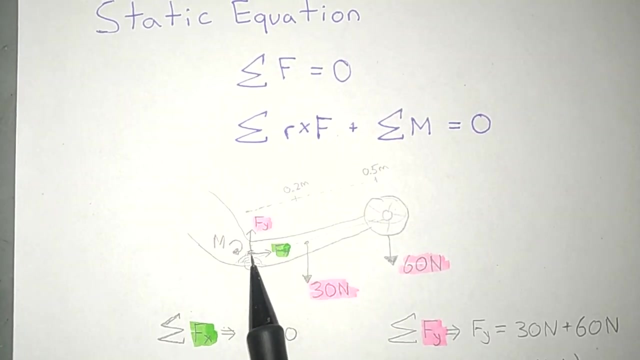 And that must be equal to. if you calculate this, you would get that the moment would be equal to the other number. Quickly, simply, quickly, important to note this point over here. sorry, this point over here is a joint. 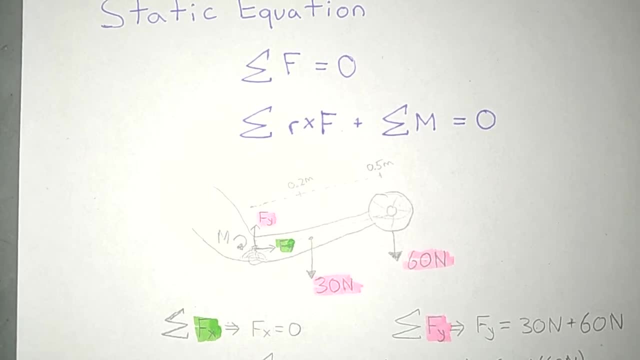 And what we usually try to do is see the joint as just a single point, That all tendons, all muscles are attached to that single point which is applying the force. But in reality the muscles are attached to a little bit in front of it. 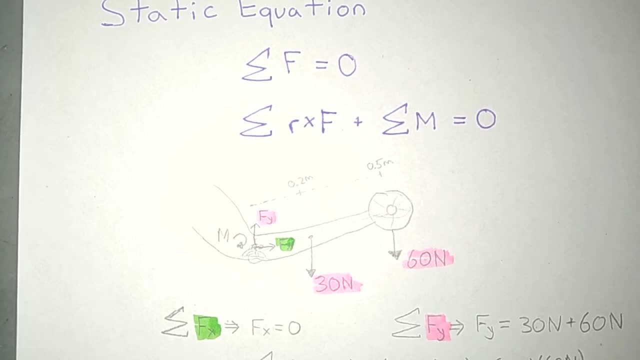 Which means that, due to the case, there's not really an internal moment being applied, especially at a ball and socket joint, And the muscle has to resist that moment. The muscle has to apply a force to produce a moment And not that the bone is producing a moment itself. 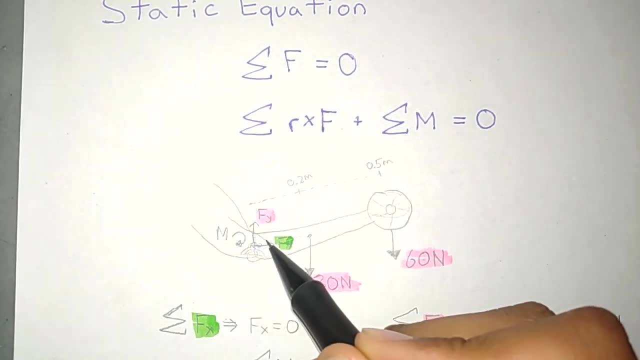 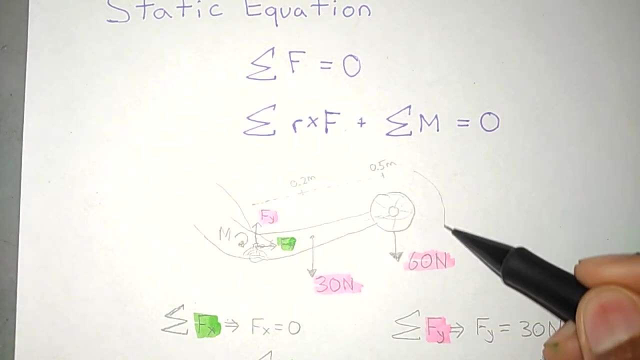 So you can see that if there's a muscle being attached over here- and let's say this was a ball and socket joint, which is in the case of an arm, because the arm can freely move in these two directions- then the arm will not be producing a moment. 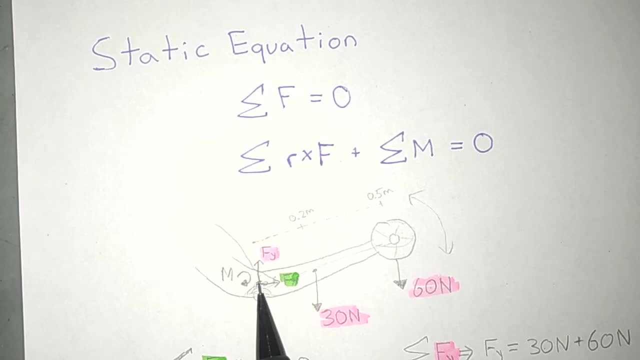 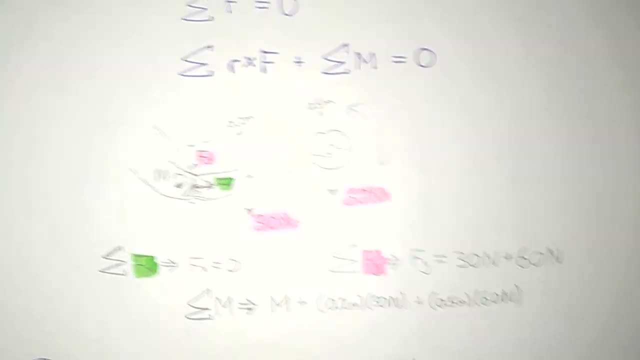 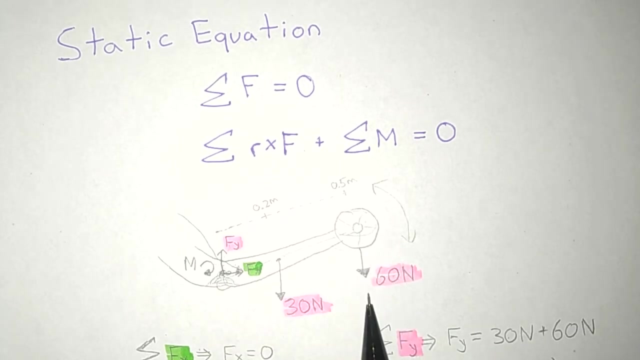 The moment that we call at the joint would actually be produced by a linear force just ahead of the joint, And if we would do the equation over here, we would see that that force must have been really great to counteract this moment being produced over here. 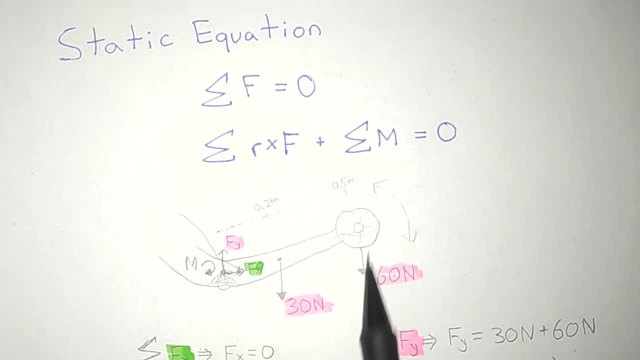 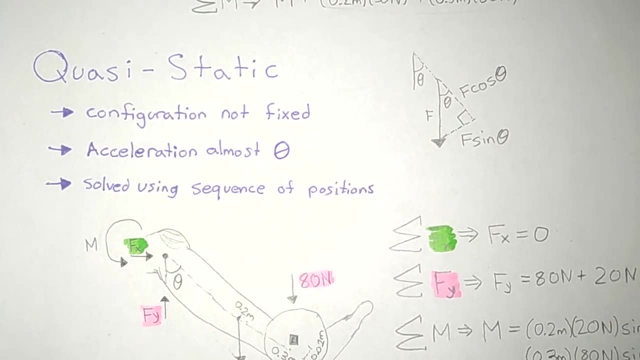 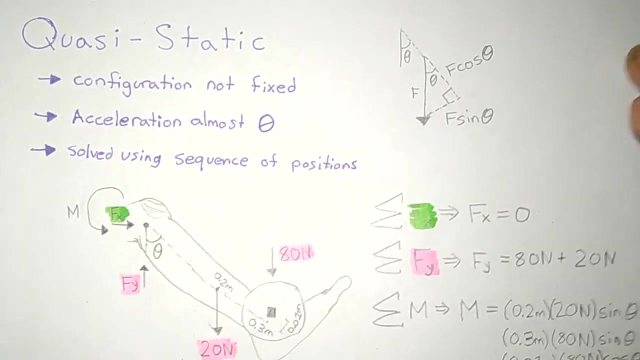 Because torque is basically force times distance, We move on to quasi-static- Quasi-static is static, static situation, but with different reference frames. In other words, the configuration is not fixed. So if we see over here, we're given an example of a person, a leg in this example. 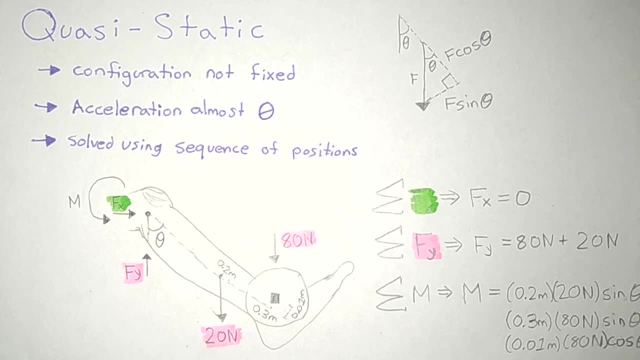 carrying a weight. But the thing here is we're not keeping the angle constant. This leg can be moving anywhere, up to here, down to here. So now, even though this is not sorry, even though this is not dynamics, in that we're not seeing any acceleration or moving. 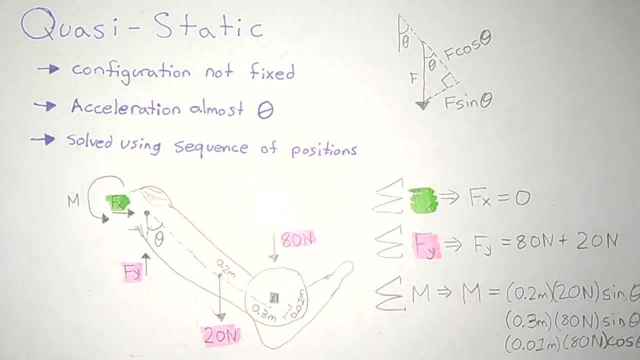 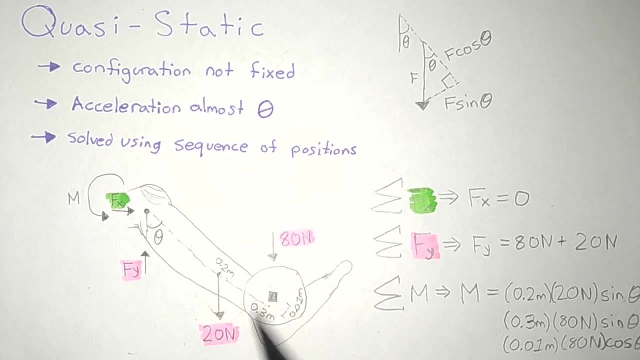 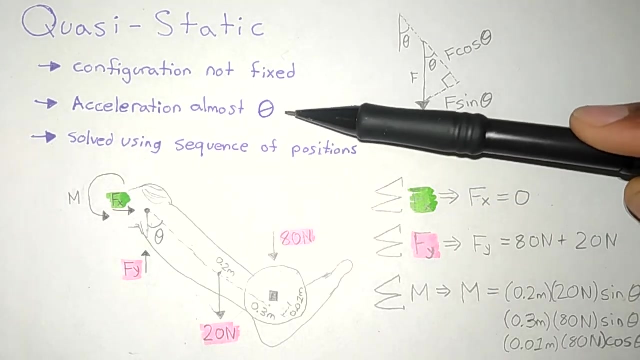 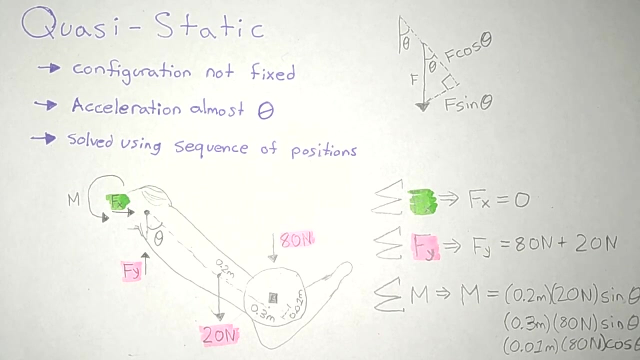 what we're trying to say is this sorry? what we're trying to say is: this force over here is not producing any acceleration. that is sorry. one second, Yeah. so what we're trying to say over here is that. 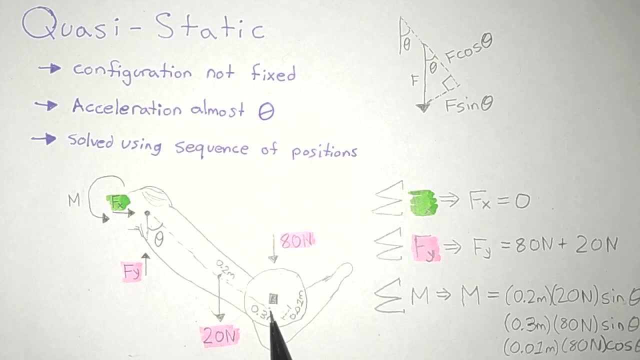 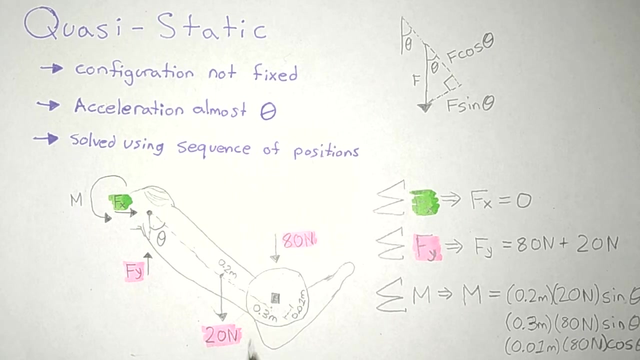 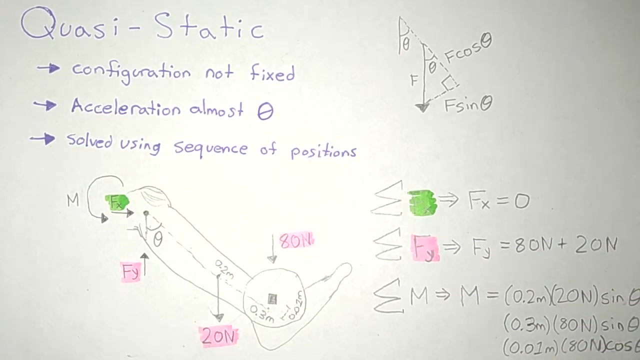 okay, in this situation we have a set frame, but we do not have the dimensions of the given points, the given forces. So, in this situation, we have a set frame but we do not have the dimensions given forces. so let me explain this. okay, so we have the sum of the X again must. 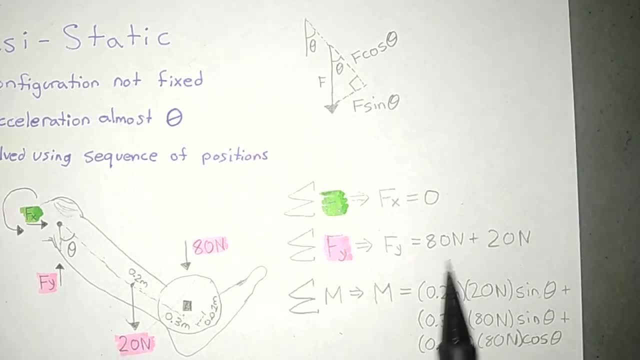 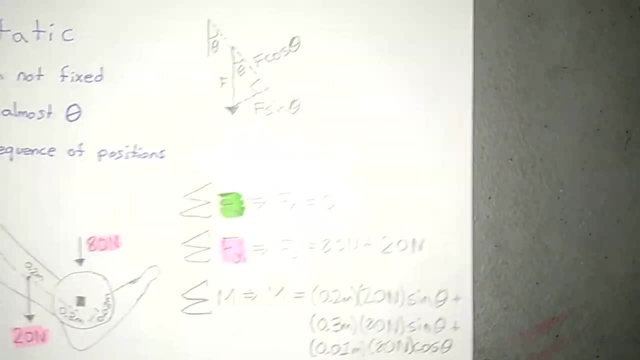 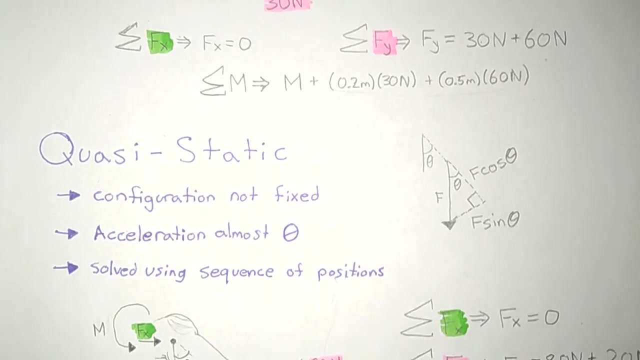 equal to 0, the sum of the Y must be equal to 0, 0 and in this case FY must be equal to the negative of these two and the moment must be equal to 0. but the problem here is, as I said, there's no sets configuration. we don't, we do not. 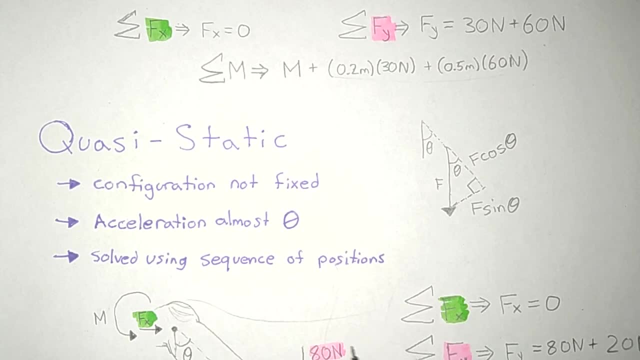 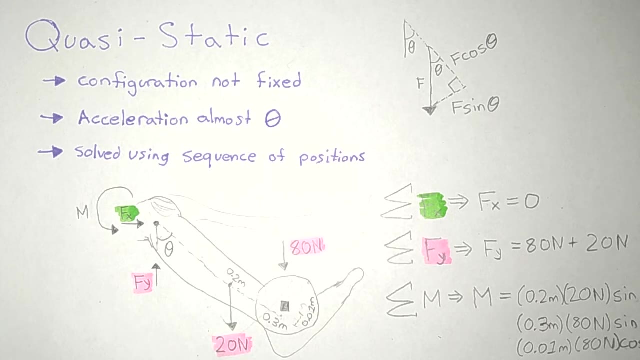 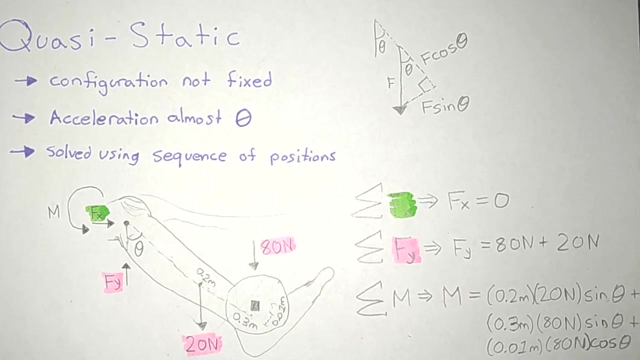 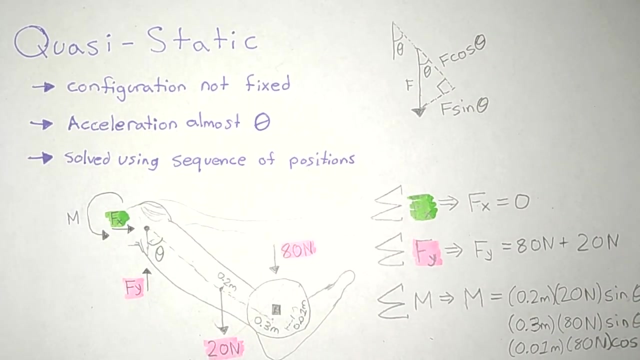 know where this weight is. this weight can easily be someone like this- I just do it like this- but it doesn't have to be in this configuration. so how would you calculate it? but we will take theta as a variable, but then you'll notice that we cannot solve the equation because it would be two unknowns and one moment two. 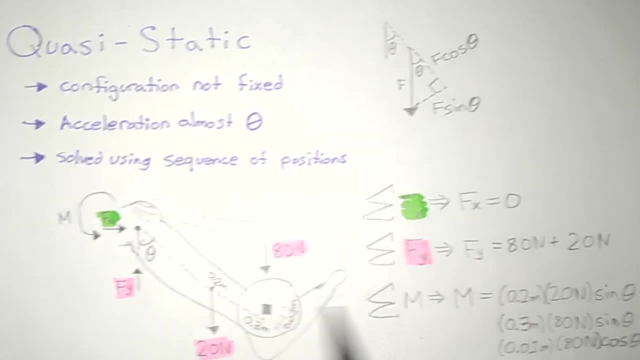 unknowns. we don't know the internal moment and we don't know the theta. even though we do know the internal moment, we don't know the theta, we don't know the x and y. that wouldn't help us into finding moment, so we're just gonna solve. 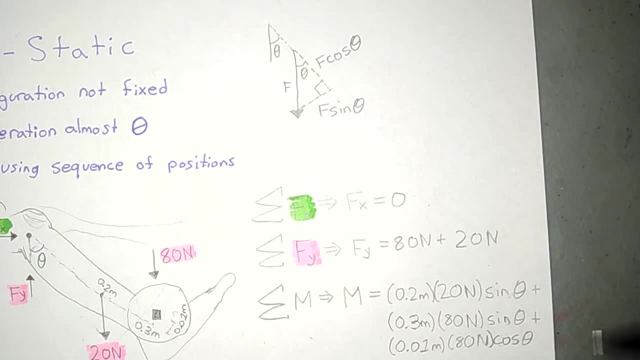 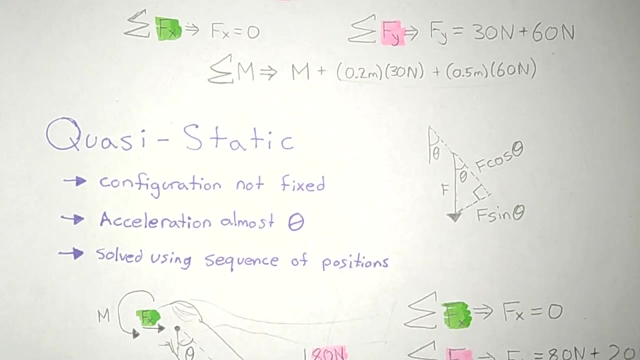 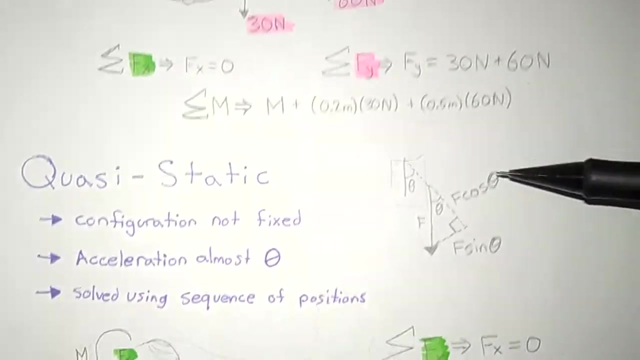 the moment in terms of the theta, which kind of makes sense. but the question is: how do you find the theta? how do you find the theta from this equation? this is going to be more mathematical. so if we say that the theta is this portion, this portion is simply this portion over here. if we say the theta is this portion, 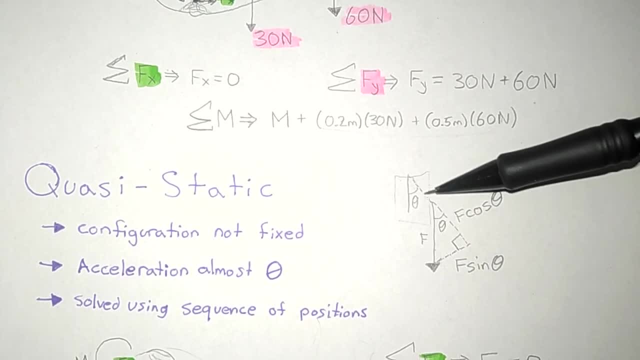 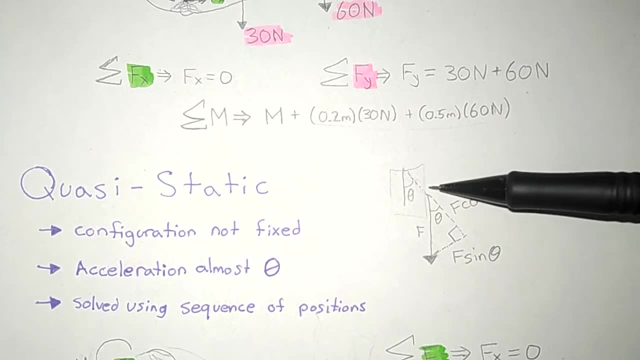 then we can extend that along the bone. this part over here is basically this whole thing over here. I'm going to extend that along the bone, this part over here. I just put it here to show mathematically. so we're gonna have a force down. let's say it's the weight, or it's the weight of the leg or the. 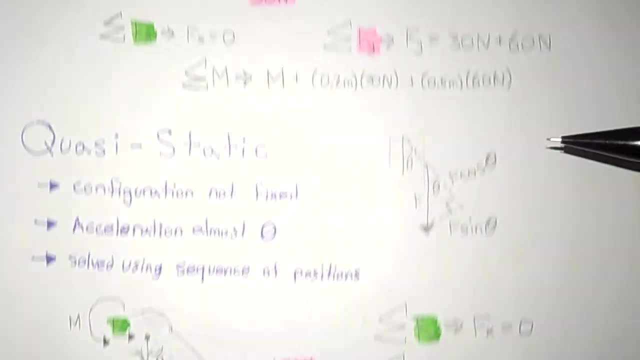 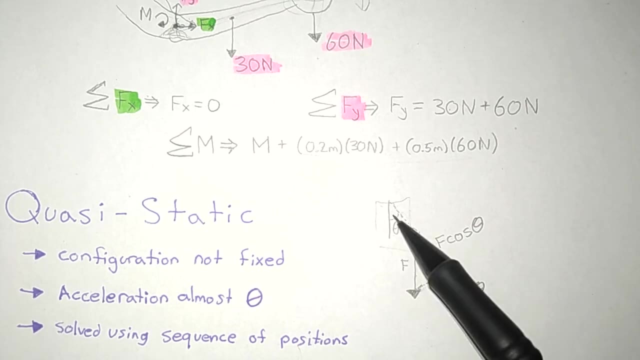 weight of the dumbbell over here. so we're gonna create a right angle triangle over here and if this is a right angle triangle, then this theta is equal to this theta, because these two lines are parallel. we have a force over here by Pythagorean- it's not Pythagorean, sorry- by the cosine law sine. 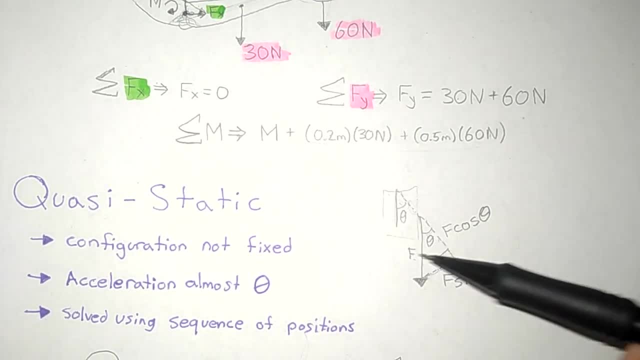 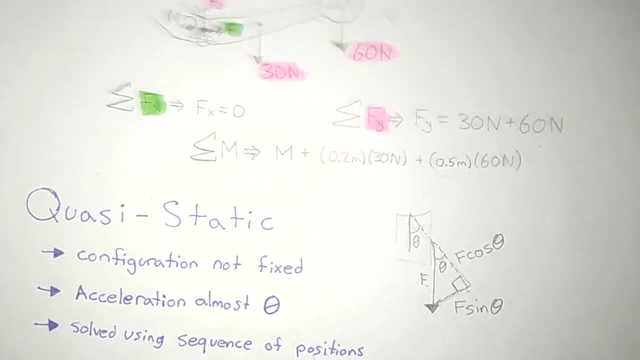 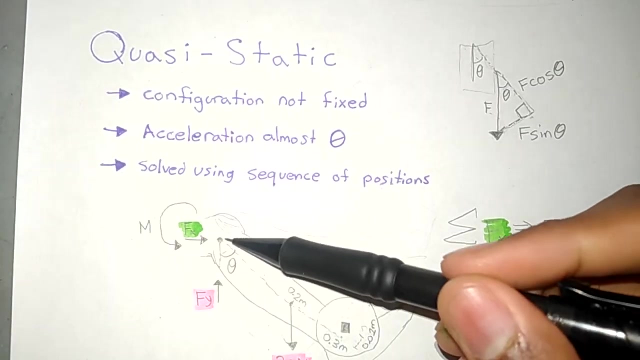 ocalypse IC. pleasant, ma we can find out that this would be forced times two- sine theta is this side- and force times cos theta is this side. okay, if that's the case, then let me quickly do this one. we have 0.2 meters up to here 20 it goes. 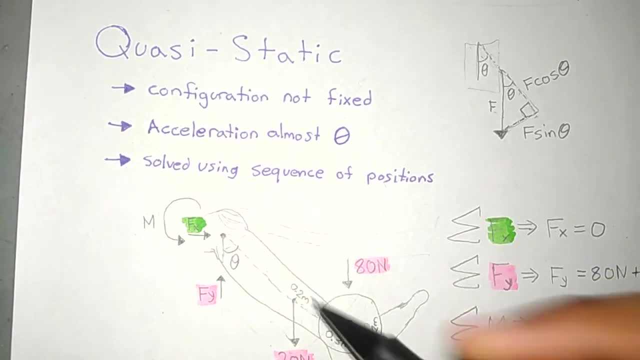 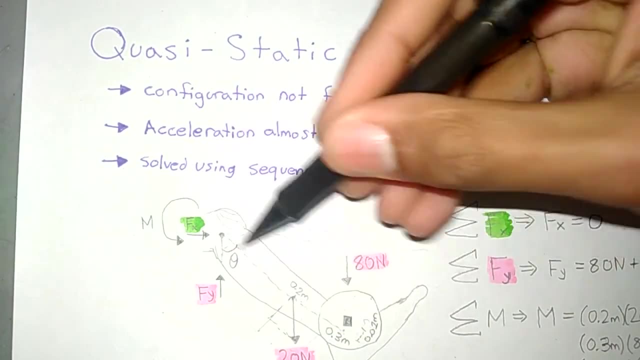 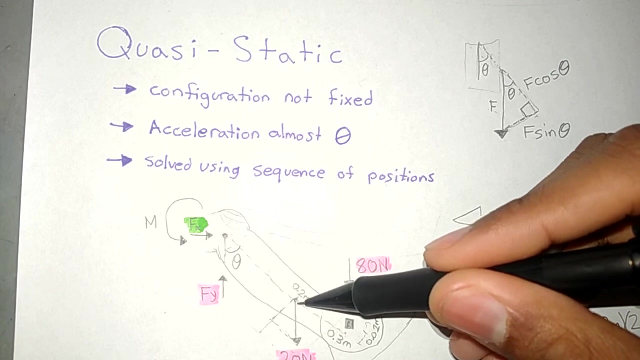 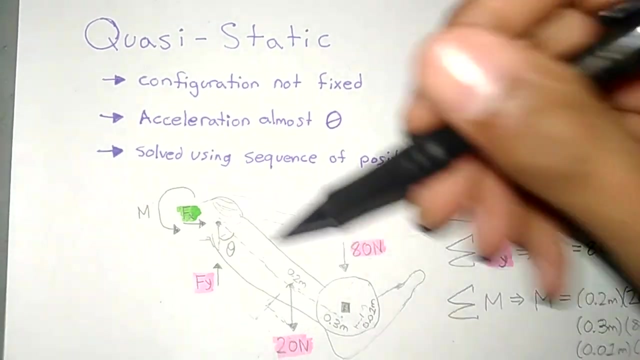 down. but what would the moment be? but what we're looking for is really this force over here. it's the only downtown That's producing the full moment. This point over here, in this direction, would have a moment parallel to the axis and perpendicular to the axis, the line. 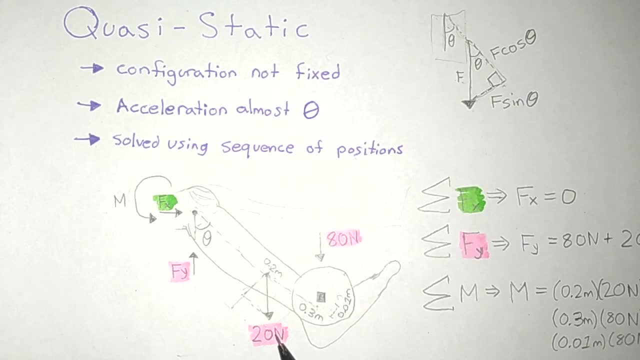 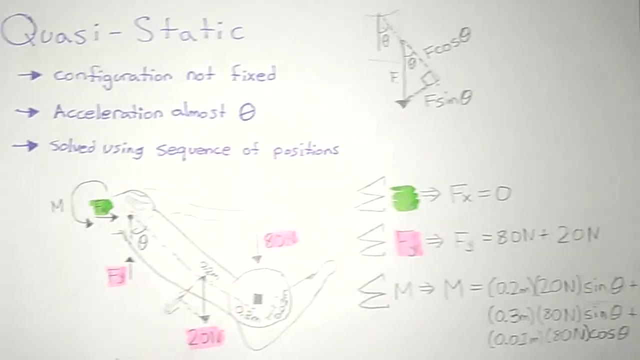 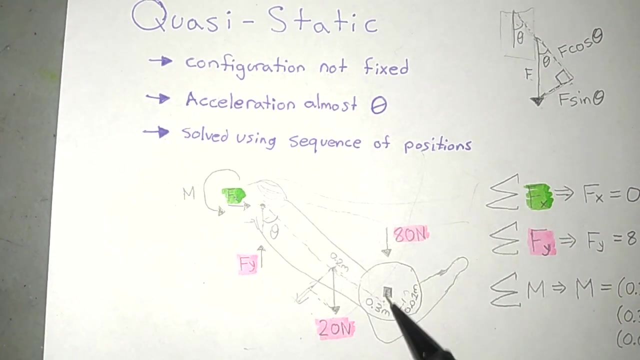 So we have 0.2 times 20, but because we have to move this 20 into this direction, we have to multiply by sine theta And we're going to do the same thing with the other two. As you can see over here, we're going to have the 80 newt comes down, but we want it in this direction, so we're going to multiply by sine theta.